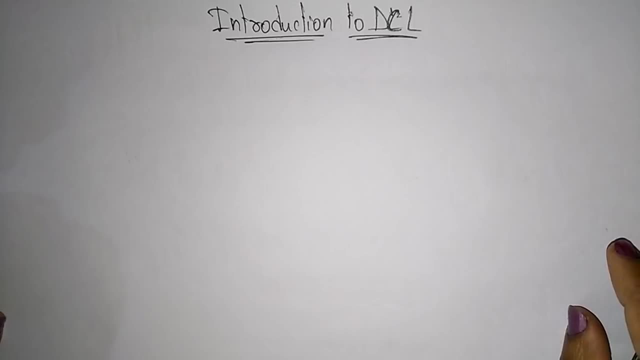 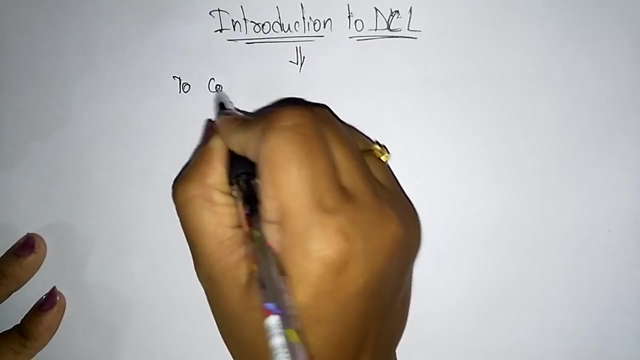 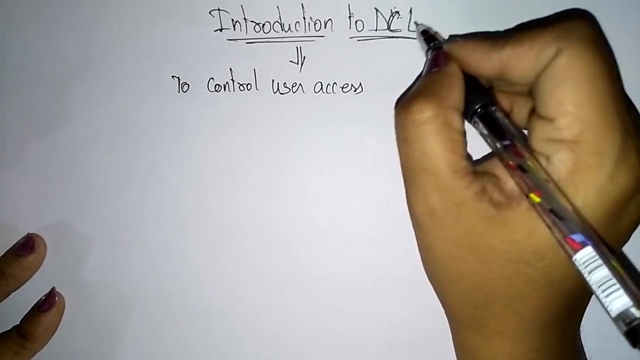 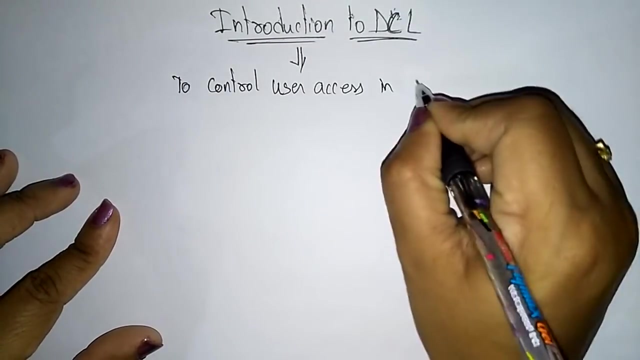 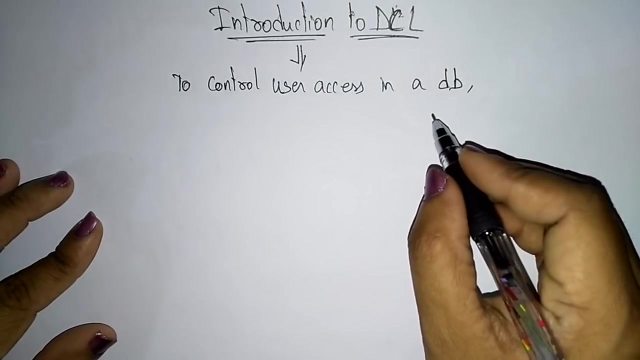 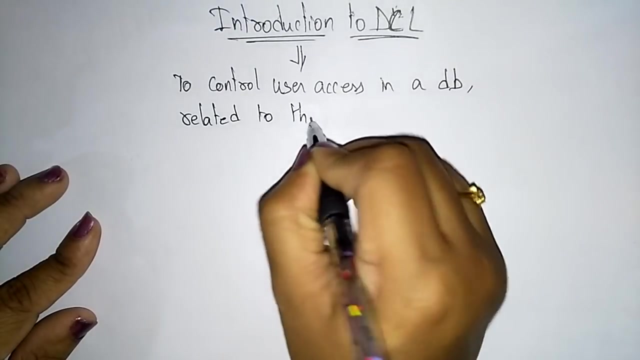 Now let us see what are the commands that are used in the data control language. Actually, the main use of this data control language is to control user access, So the name itself is indicating this language is mainly used for controlling the tables, So it control user access in a database And related to the security issues also Why we are controlling the database. Related to security issues. 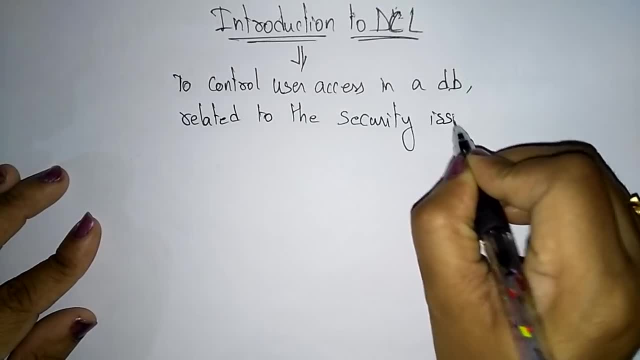 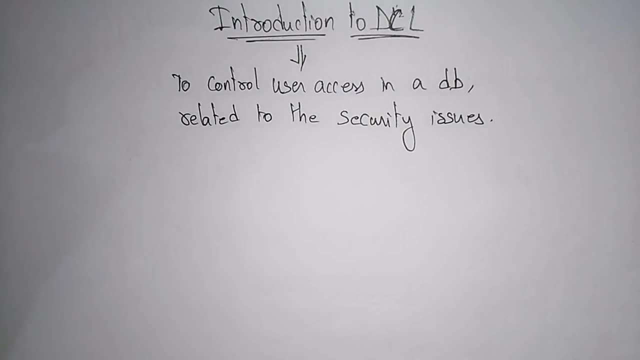 So the main use of data table is to maintain the records securely and the huge amount of data that wants to be stored that can't be use by the files. So instead of storing the data in the files, we will use databases to store the data. 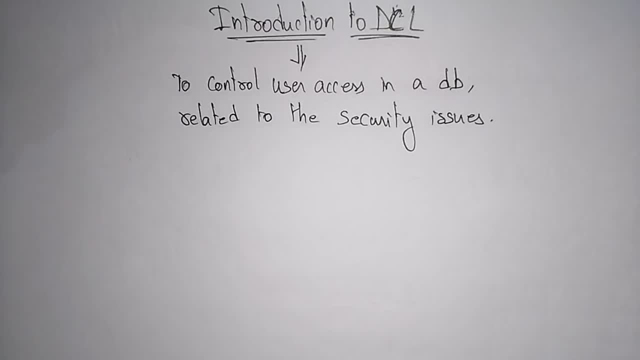 So if we want to store any data, you need some security. So without security we can't。. But if we want to store any data, you need some security. So without security We can't. You can't put the important data that is related to the organization Okay, So further, you need some security access. So this control language, data control language, is used to control user access, means the person who has the permissions to view the database or to modify the database. that person can only enter the database. 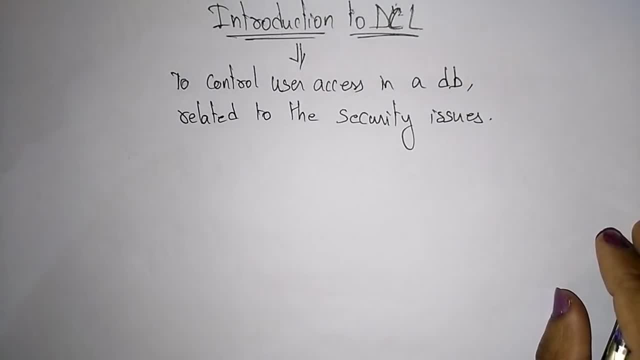 Means he can access the database. Okay, So for that you need some permissions. So the permissions will be given by the administrator who is created, the monitoring, the complete entire database. Okay, So with the help of the username and the password, every user can access the user who has given a permission. that user can access with the help of username and the passwords. 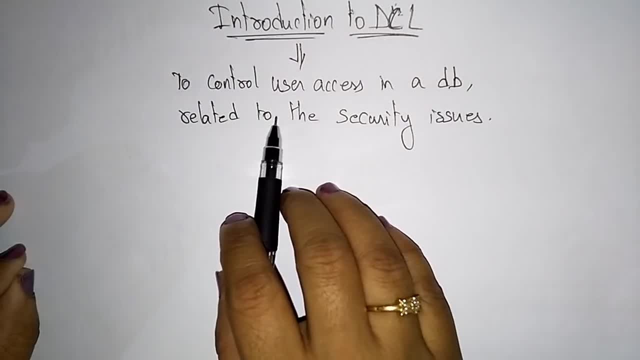 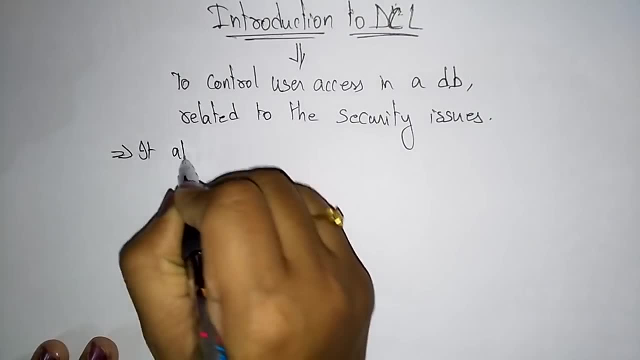 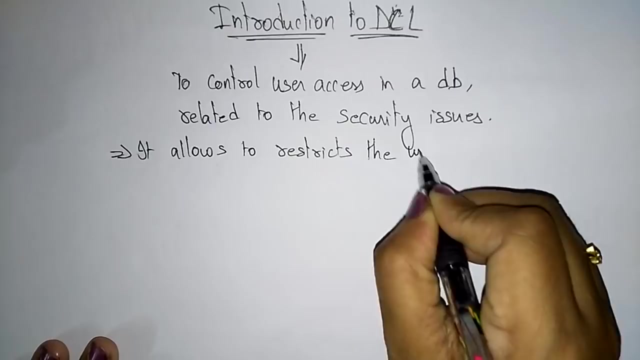 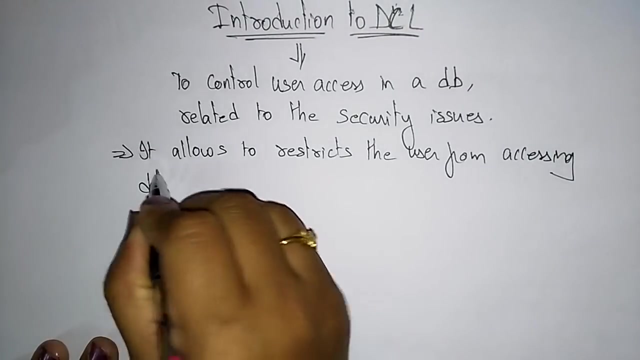 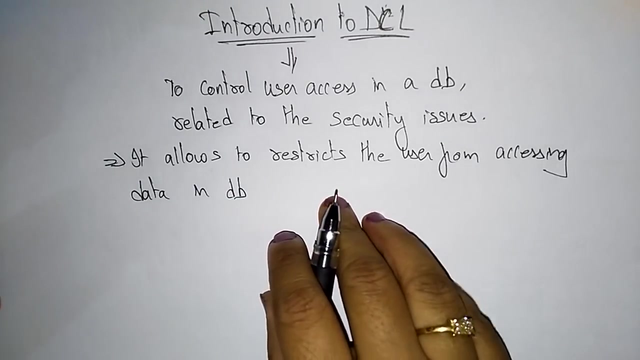 So those username and passwords are nothing but the controls Control user access. It allows to restrict, restricts the user from accessing data, accessing data in database schema. So that I said so. the main use of this TCL is to allow the restrictions to the user from accessing the data in database. 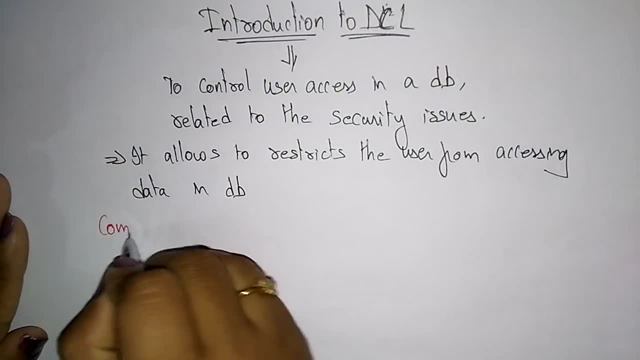 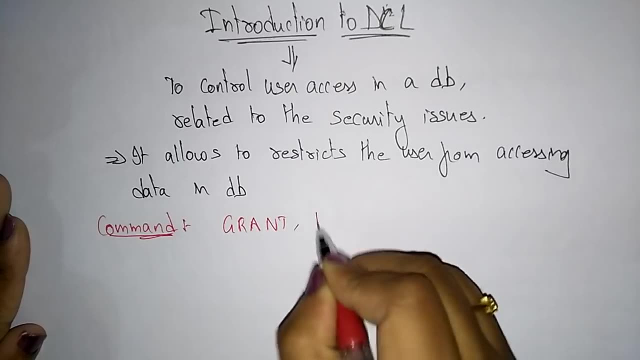 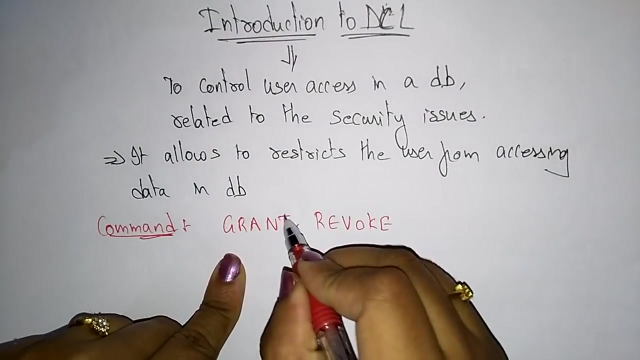 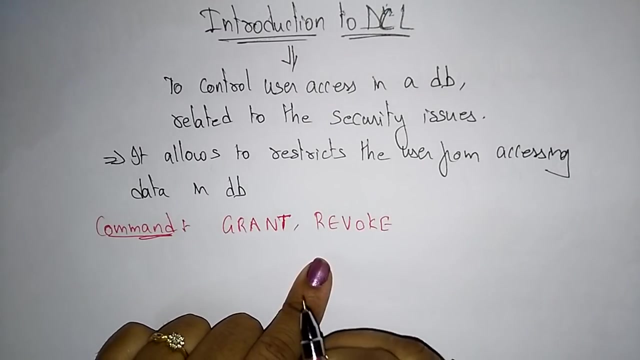 Now what are the commands that are used to control the user access? So those are the grant and revoke. So the names are saying that grant means the administrator is granting the permission to the user to access the database, whereas revoke- revoke means releasing the permissions, means if the person is 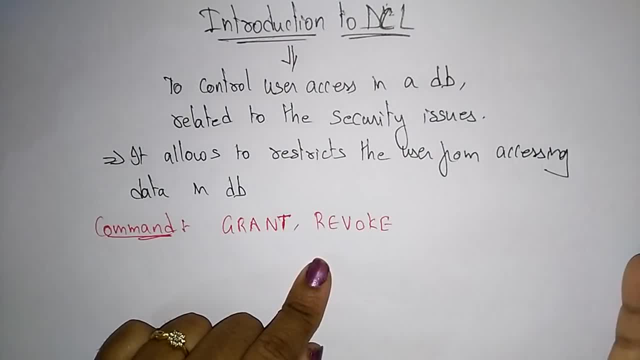 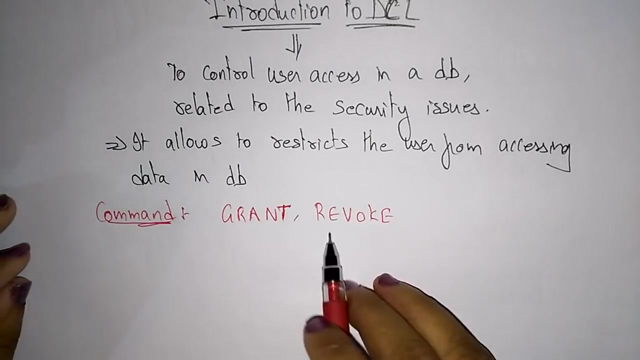 About to quit the organization, you have to release the permissions to access those database means you you're updating the control. access means you're updating the usernames and the passwords and you're giving permissions to the another with the help of the revoke. so grant is giving the permissions. 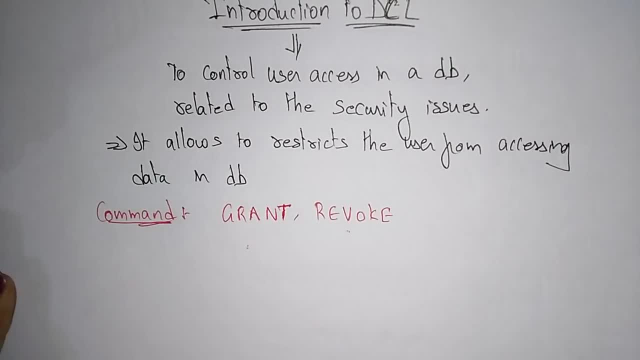 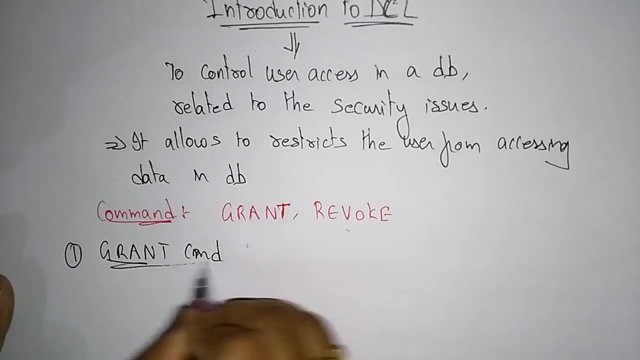 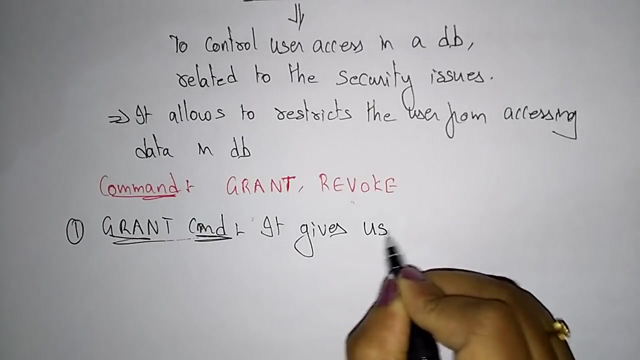 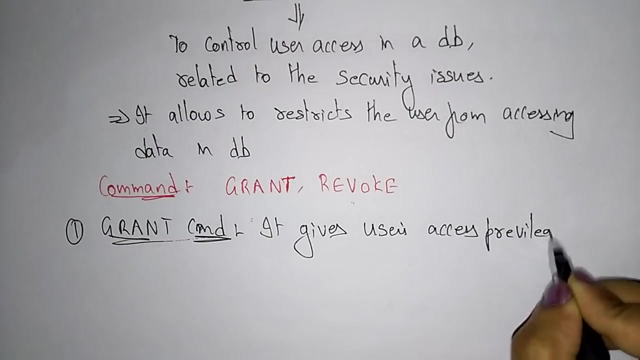 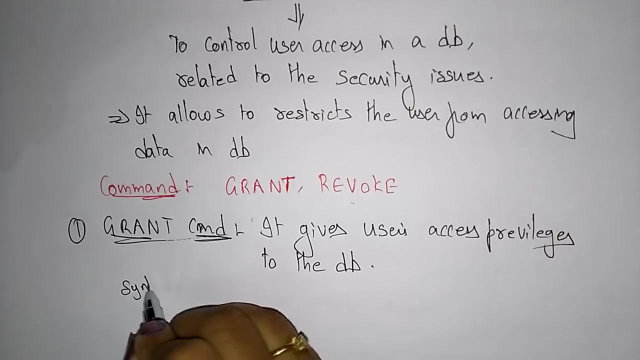 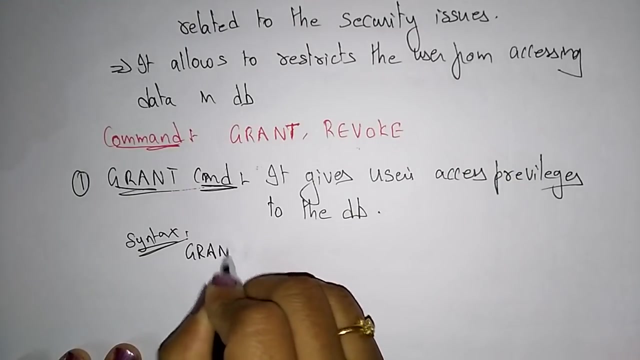 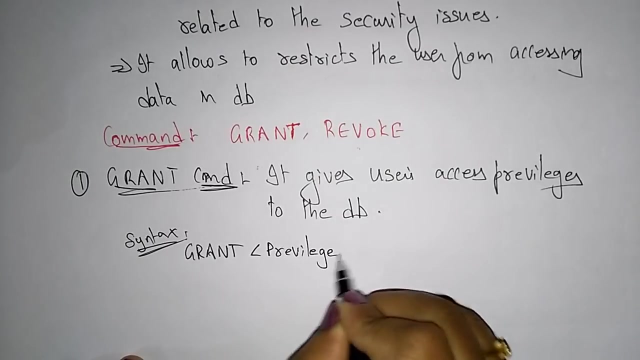 revoke means releasing the permissions. so now let us see what is a grant command. the grant command? it gives user access privileges to the database. the syntax for this is so then, what will be the syntax for this? you had to write the keyboard command grant. next, the privilege list means your. you want to act, you want to allow the person to. 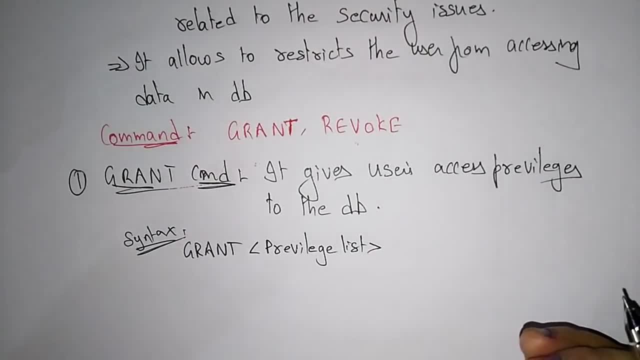 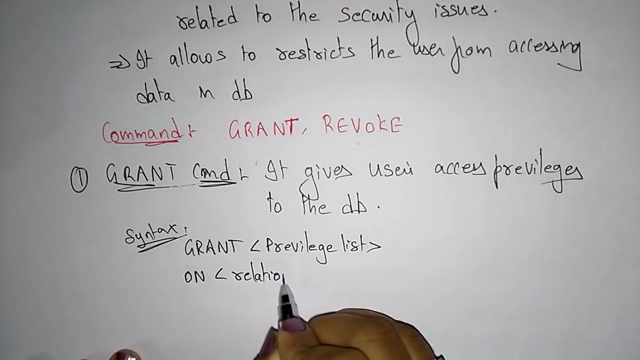 access complete database or you want the. you want to allow the permit. allow the person only to view particular rows in the table. okay, particular fields in the table, only particular table in the database. so that is a privilege list. grant privilege list on relational name. is table name, relation name or view name? 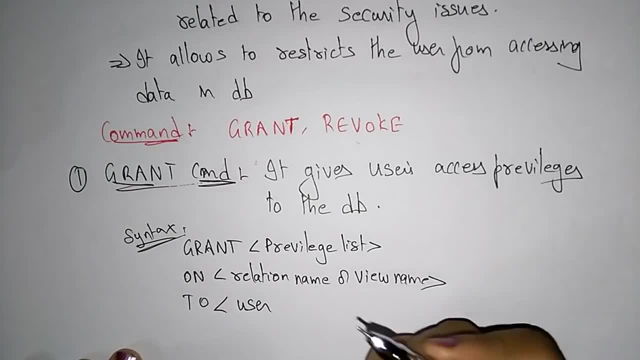 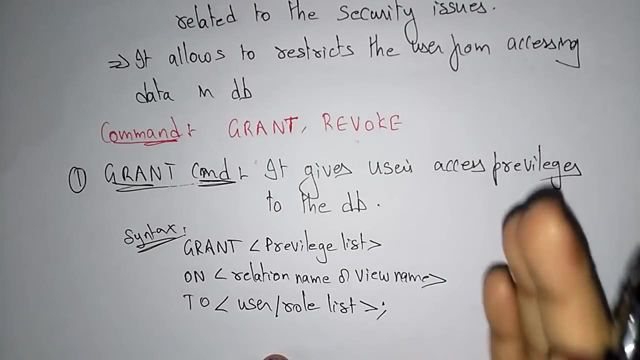 to the person to whom you want to give the permission to access the database. so this will be given by the. this grant permission will be given by the administrator who is accessing, who is having the control on database, the complete privileges, that is, that are there for person. 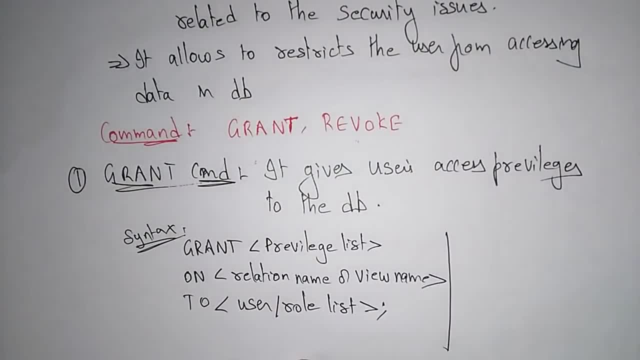 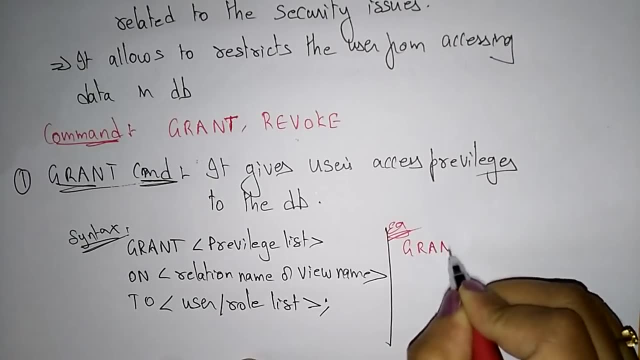 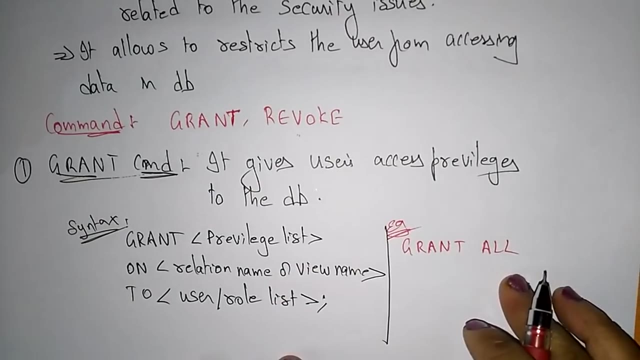 that person can give this privilege. now let us see the example for this. so here i am: grant all. so the privilege list here i'm saying as all means the user can access complete database, grant all on emp elementos, all on emp dimensions. like this i have the privilege list because the counter used is alwaysم wel variation, because the under retrieving or handling is always�ก Year 1.0. 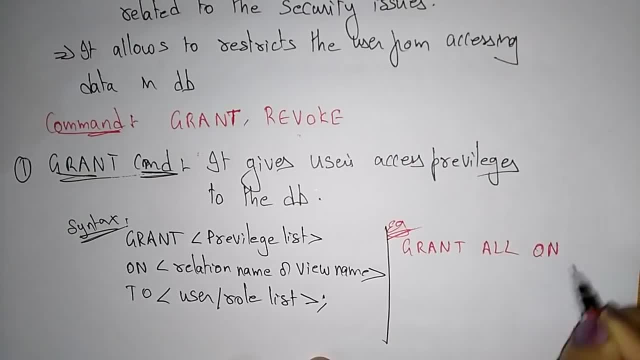 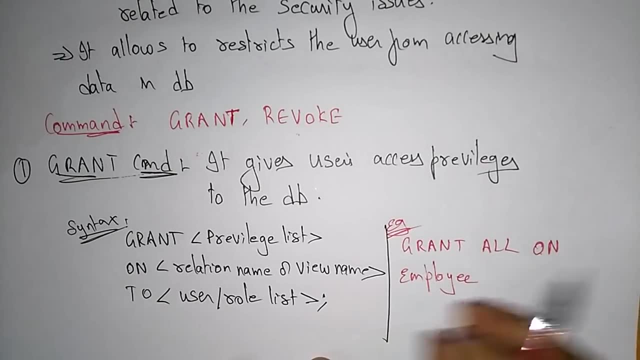 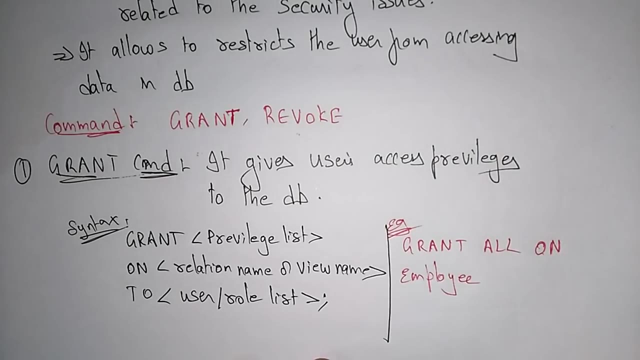 the user can access complete database brand all are employees of all all means. the user can access complete database grant all on employees and remaining users must have you Grant all on employee. So only on employee, Only on employee table. he can do all the fields Means he can access all the fields, He can update all the fields or he can change, he can do modifications on the tables. 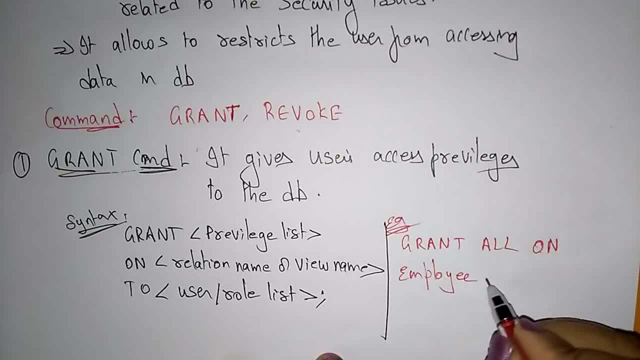 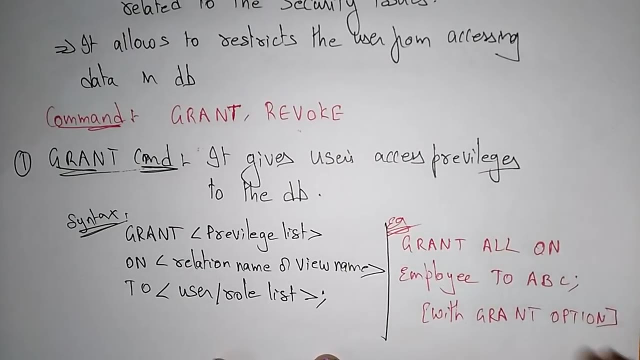 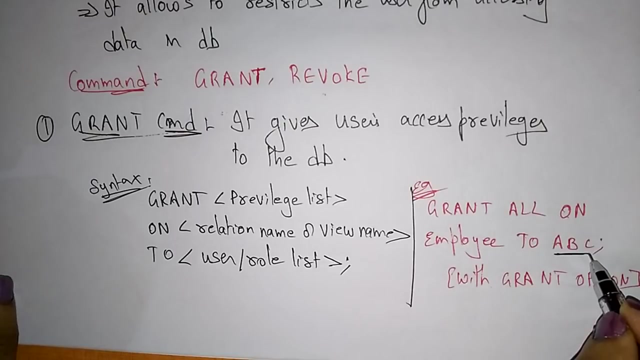 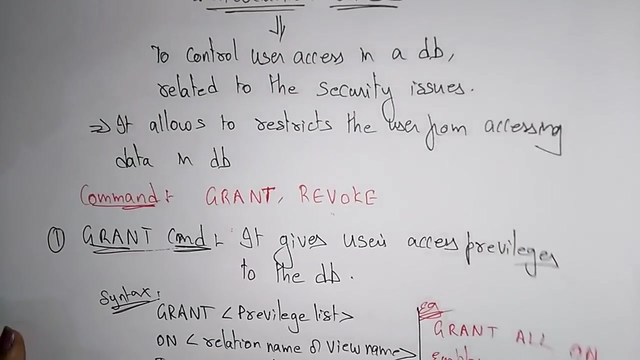 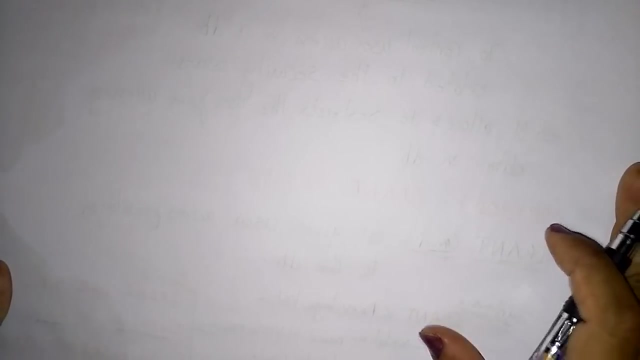 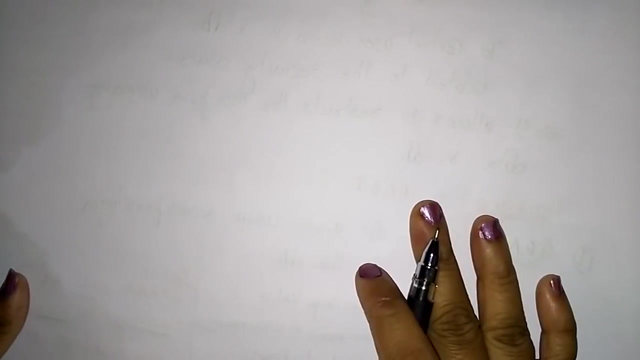 Employee table Grant all on employee to ABC person. Okay, So with grant option. So this is a syntax. So here user ABC has been given permission to view and modify the records in employee table. So this is about the grant. Now let us see the next command, that is, revoke. So once the user has given a permission to ABC to access the employee table, Means now he can update the table, he can delete the table or, if you want, he can modify the table, He can insert the values in the table whenever he has given the permission. on employee table. 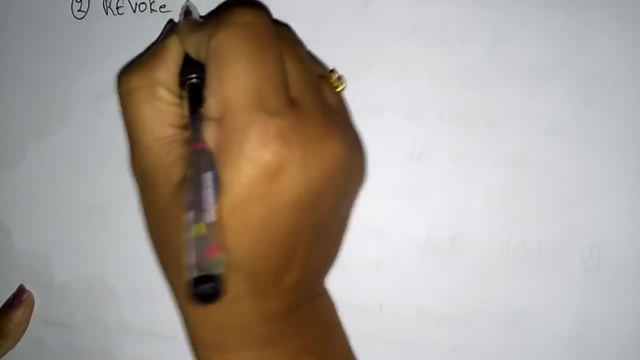 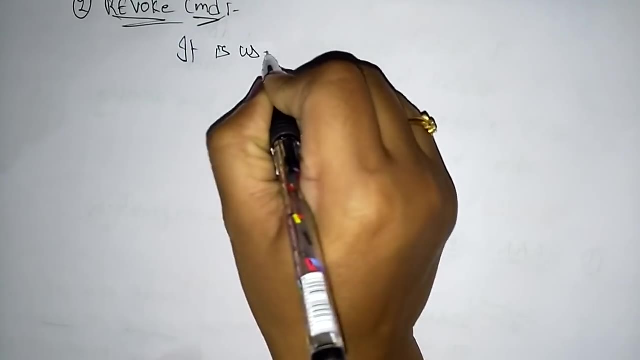 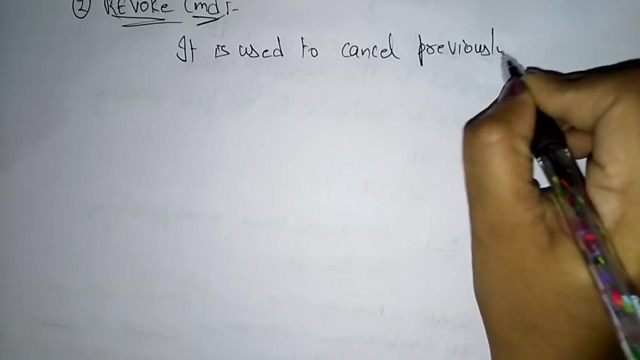 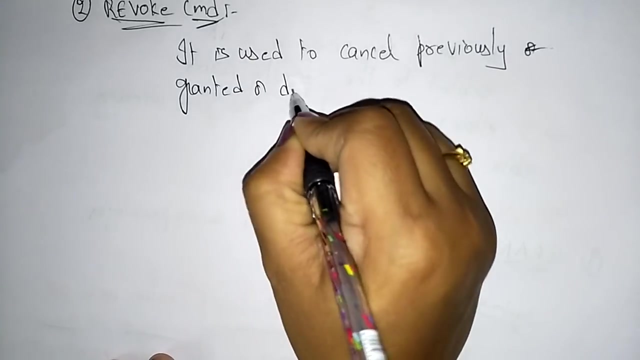 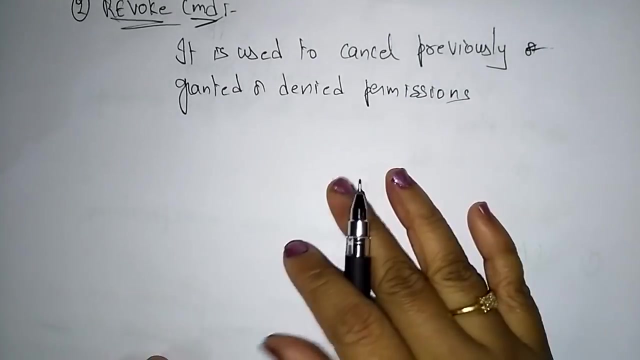 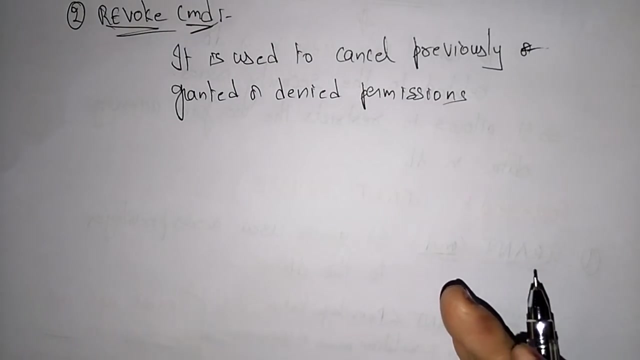 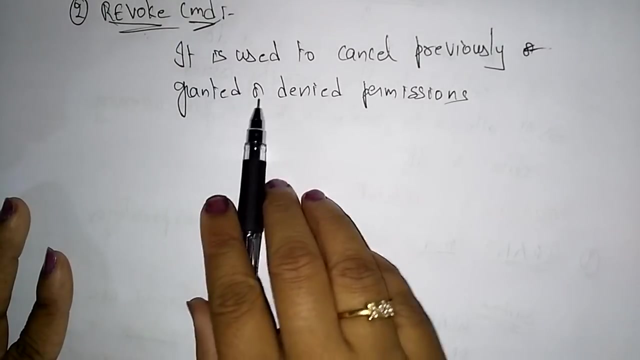 Now the revoke command. What this revoke command will do. So it is used Use it to cancel previously granted, Previously granted or denied permissions. So the revoke means So previously I granted a permission to the ABC, Now I can cancel the permission to that ABC person. So this revoke command is used to cancel previous granted permission or denied permission. 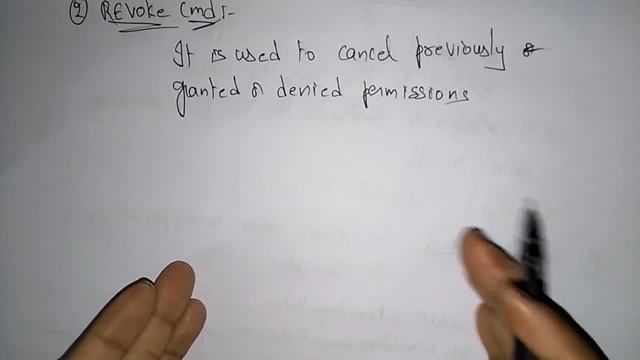 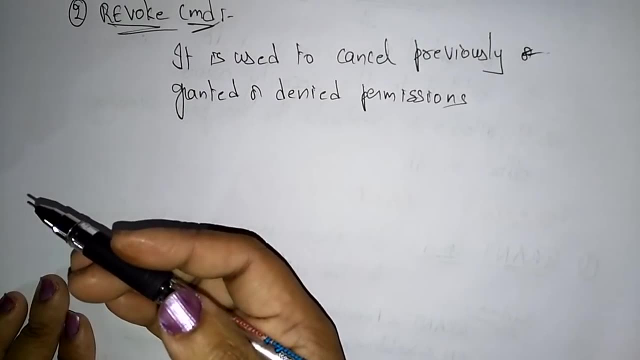 So suppose you block one person. Okay, Suppose if you want to give the permissions to that person, you can give by with the help of the revoke command. So all the denied permissions will be released and he can granted that person can granted to access the database with the help of the revoke.